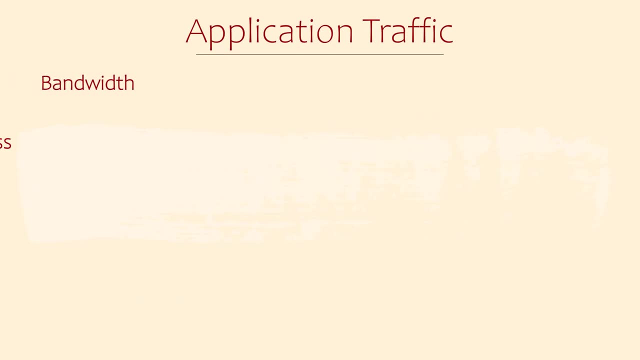 web page can offer. In particular, we want to look at bandwidth loss, latency and jitter In networking. bandwidth refers to the amount of data that needs to be transferred. We measure the maximum bandwidth of a link by the maximum number of bits per second that it can transfer. 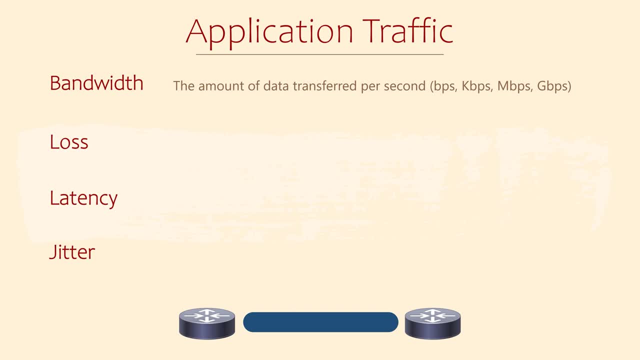 Some applications, such as video streaming, need a lot of bandwidth. Others, like using SSH to manage a router, need very little bandwidth. Loss is where the traffic does not reach the destination. There may be several places along the network where traffic can be lost. 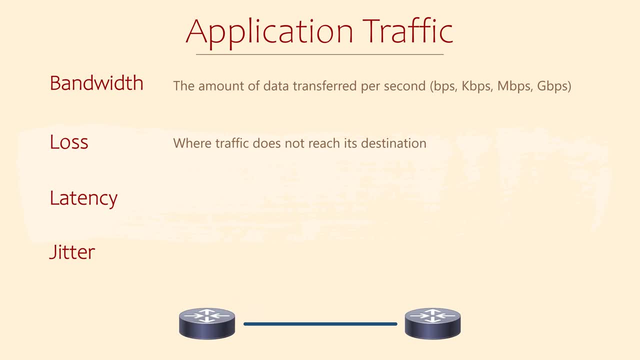 We measure loss in the percentage of packets that didn't arrive. For example, if we send 1,000 packets and 990 arrive, then this link has 1% loss. Latency is the amount of time it takes for a packet to travel from one endpoint to another. A similar term: round trip time. or RTT, is the amount of time it takes for a packet to travel from one endpoint to another, For example, for a battery to be transferred from one port. it is the amount of time that it takes for a battery to reach another port. 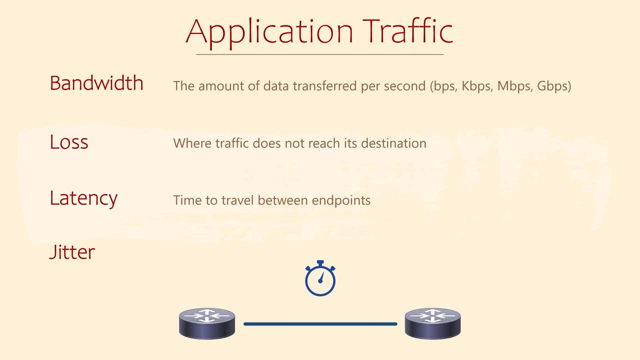 Contrary to the experience of using an LPGA, it is the amount of time it takes to transfer the battery from one port to another. That is how something can not be transferred, as you can see by the length of the pipe, It is when the battery is not studying the power of a battery. 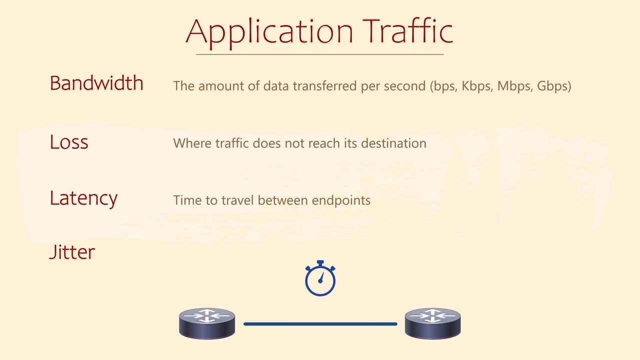 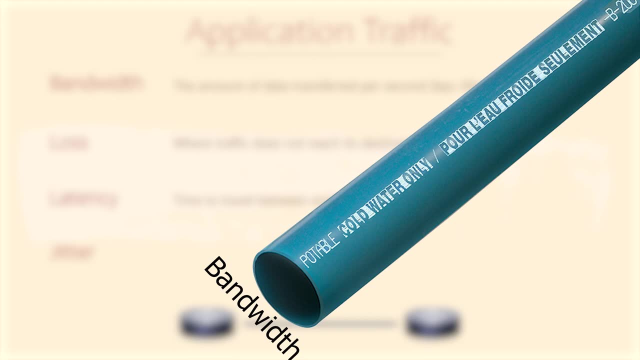 There are several other applications where you can compare those to each other. First we will look at latency. Latency and bandwidth are sometimes confused. Imagine it like a water pipe. The bandwidth is how wide your pipe is and it controls how much water can fit into the pipe at any. 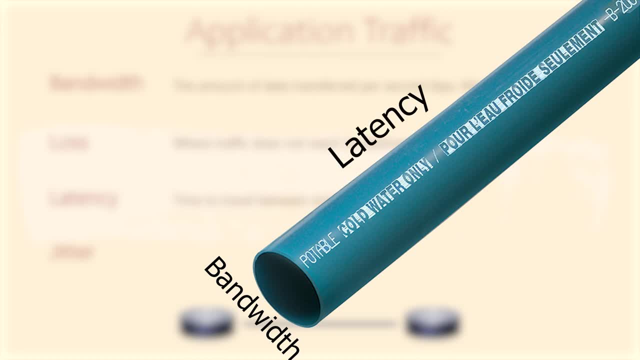 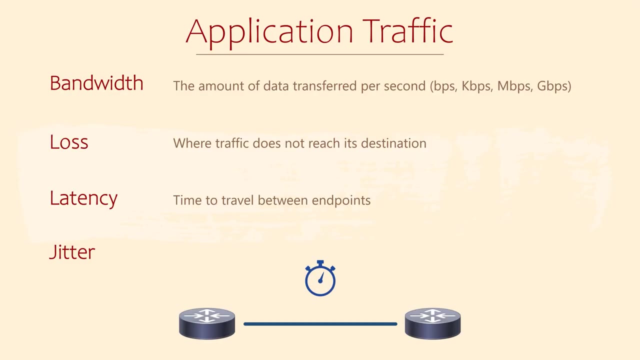 time. The latency is like the length of the pipe, which affects how long it takes for the water to travel down the length of the pipe. Applications like HTTP are very tolerant to high latency. Others, particularly real-time traffic like voice and video, are more latency sensitive. 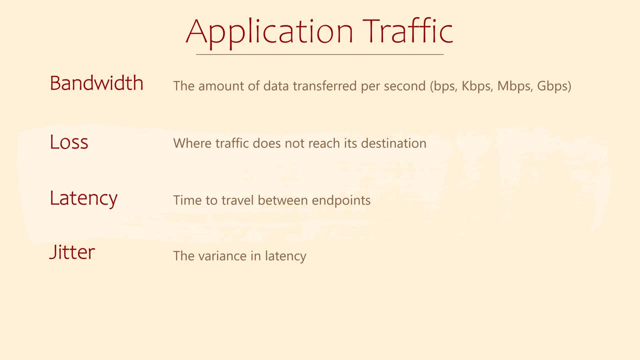 An interesting one is jitter. This relates to latency. Latency measures the time for a packet to travel between two endpoints. Jitter measures the variance in this time. Imagine we measure the latency of five packets. Delivery takes 10 milliseconds, 20,, 7,, 55, and 37 milliseconds.